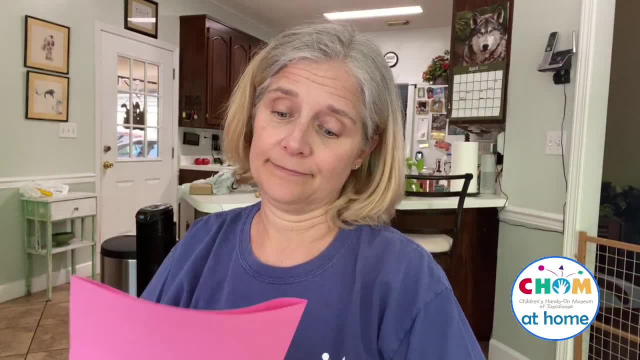 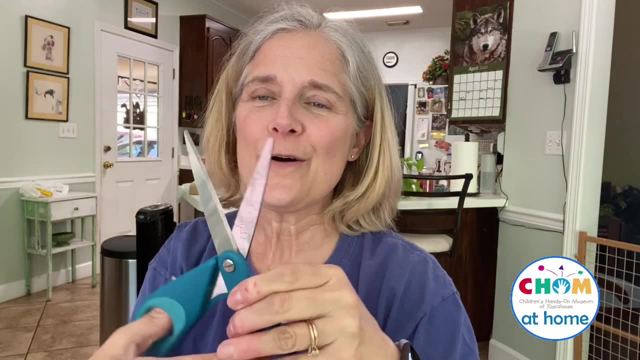 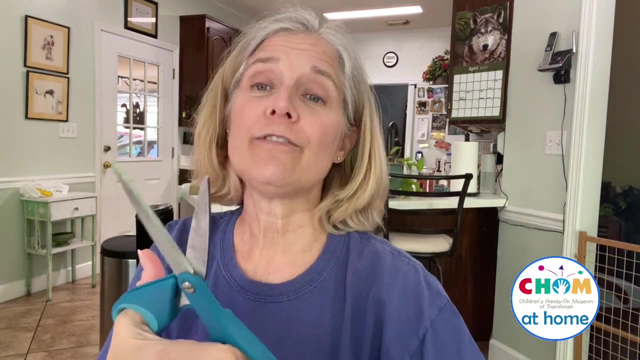 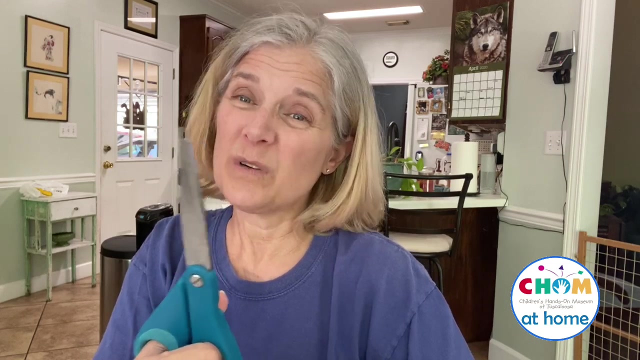 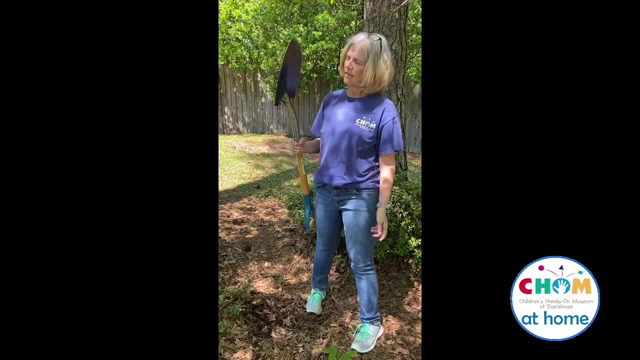 Wedges. Wedges cut things. See how each blade is really an inclined plane and they have to move in order to do their work. unlike an inclined plane that stays still when you use it, Wedges can lift or move something. The wedge on the bottom of this shovel is actually made of two inclined planes and they 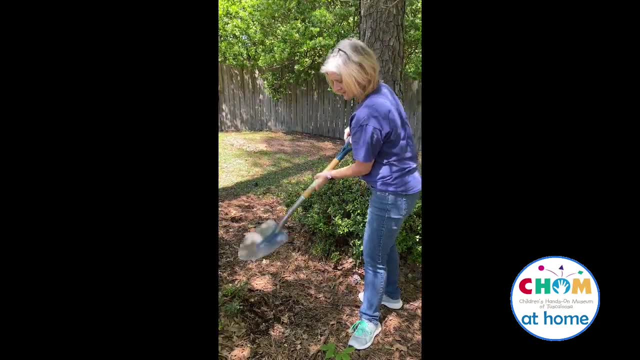 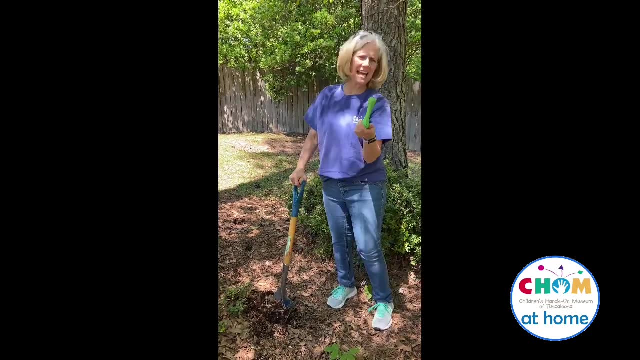 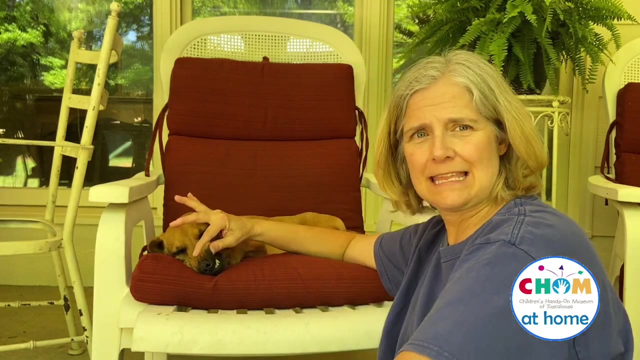 are kind of curved inclined planes. What is, Lena, Your bone? I know what else is a wedge, Somebody's sharp baby teeth, Because this week they chewed a hole in one. Oh, That was the best scratching we ever saw out. 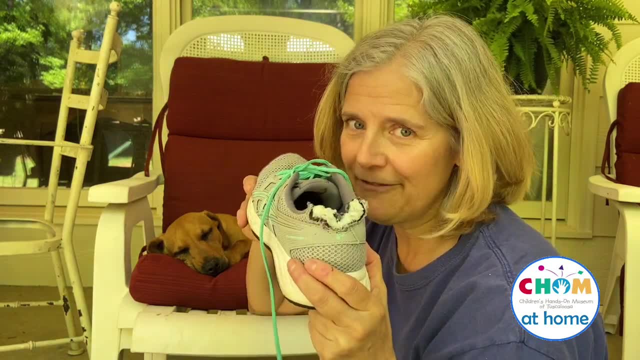 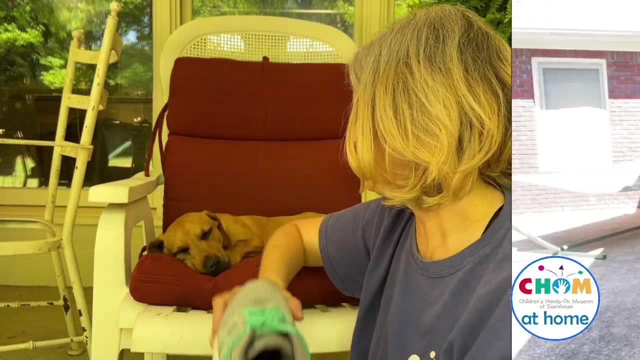 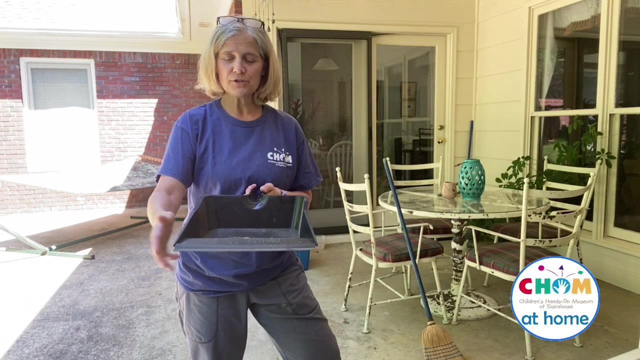 of our year. hole on the back of my tennis shoe- Definitely a wedge. They cut right through my shoes- Awesome. A dustpan is a good example of a wedge When you lay it on the floor while you're sweeping. this straight edge right here is actually. 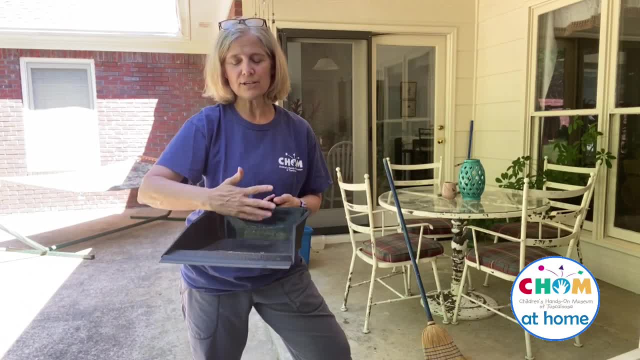 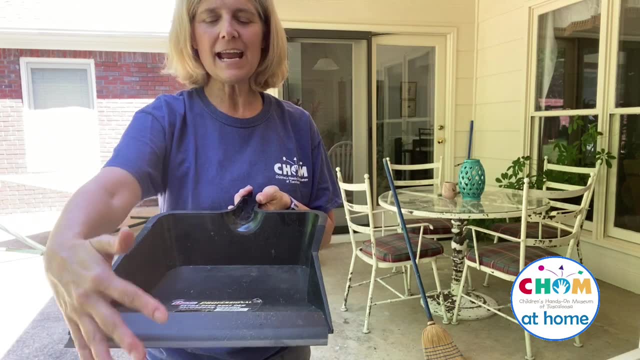 wedged against the floor so that when you sweep the dirt and the trash it goes right in the dustpan. Also, there is an inclined plane right here, just like all wedges have, so that the dust and things will go in more easily. Now I'm gonna. 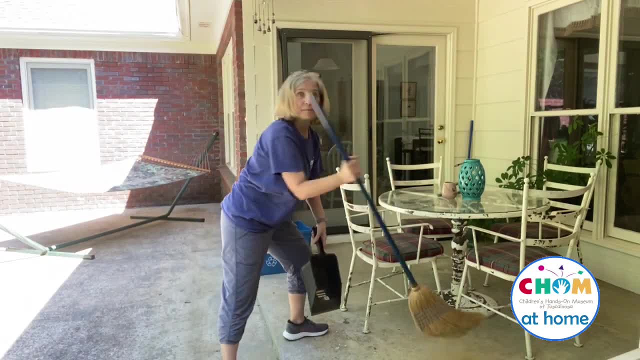 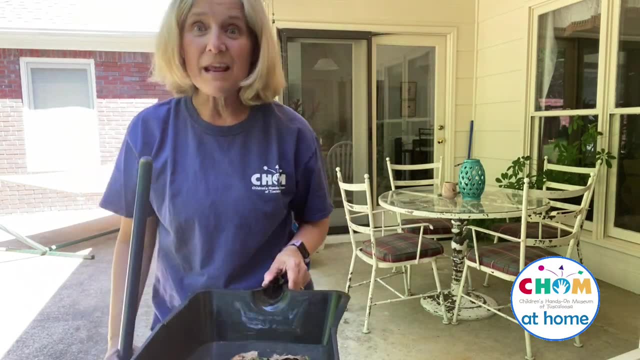 sweep up a mess over here and you're gonna notice that I'm gonna have to move the wedge to keep collecting it, Because wedges are an inclined plane, but you have to keep moving them to make them do their job. That's much better. 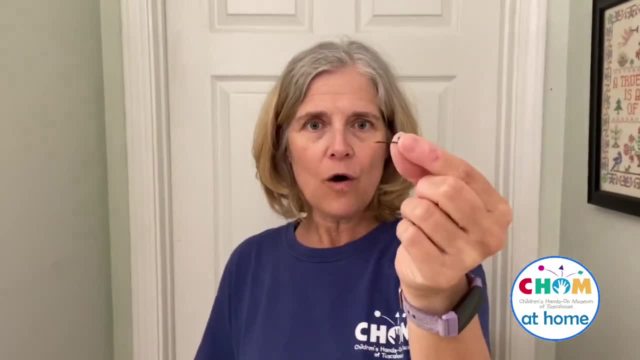 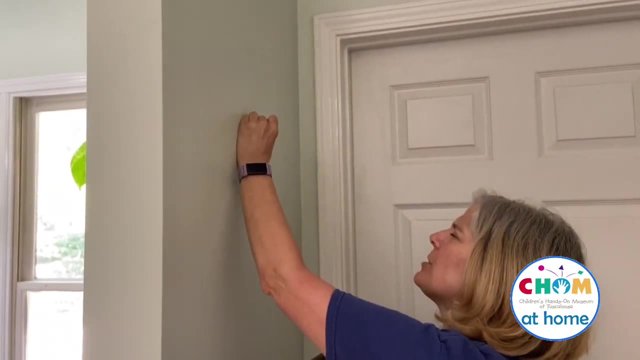 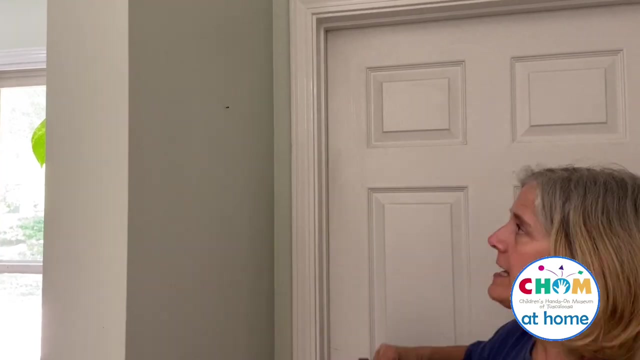 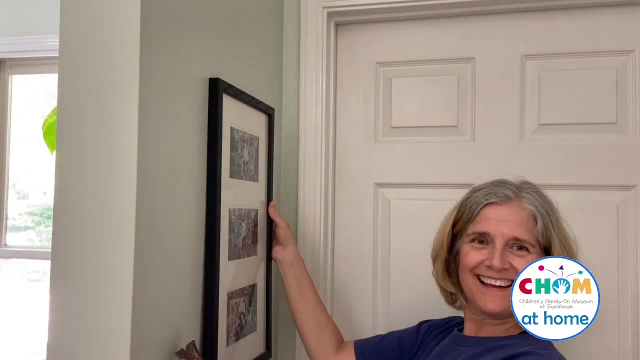 Wedges can actually bore a hole in the dustpan In something. This is a picture hanging nail, So put it There we go. So I bored a hole in the wall and attached the nail so I can hang this picture. Ta-da Well, now that you know.